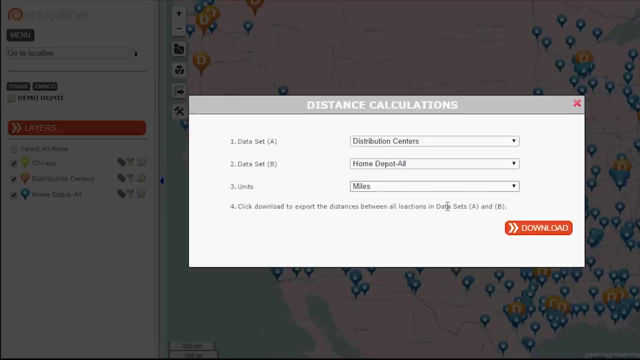 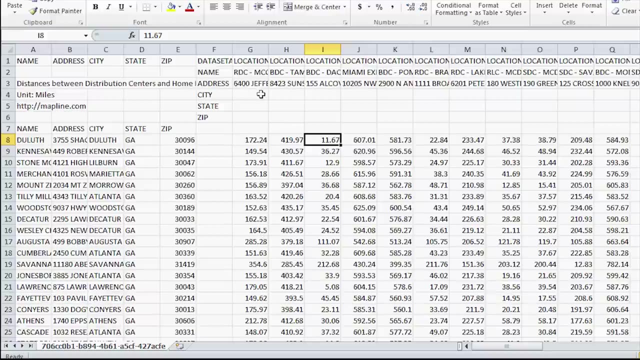 Here I select which datasets to use. I click download. Once I do that, an Excel sheet will come up having the distribution centers on the top and the retail stores down on the side. So if I want to know the distance from this distribution center to this store, 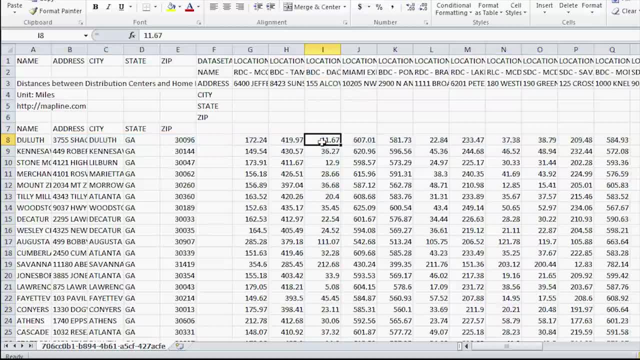 the answer is right here, And that's how you use the distance calculator. 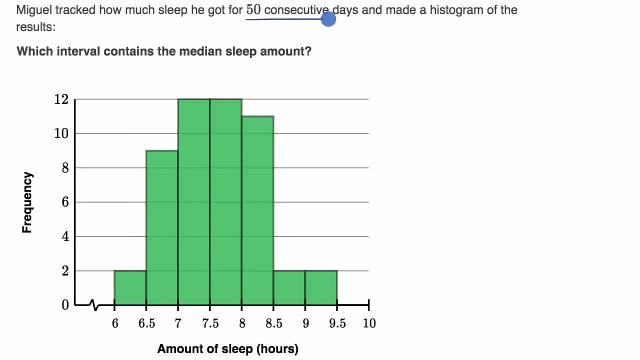 Miguel tracked how much sleep he got for 50 consecutive days and made a histogram of the results. Which interval contains the median sleep amount? And so they're saying: is it this interval on the histogram from six to 6.5, or this one, or this one or any of these? 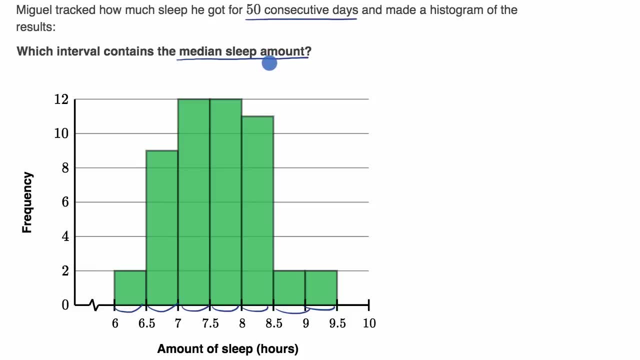 Which of these intervals contain the median. Pause this video and see if you can figure that out. All right, now let's work through this together and let's just remind ourselves how we find the median If I had the data points 11, nine, seven, three and two. 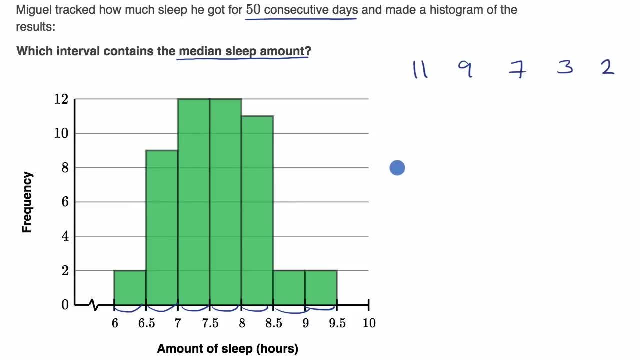 the way that we find the median is. we can order it from least to greatest, or actually you could do it from greatest to least, but let's do least to greatest. So two, three, seven, nine, 11.. And the median would be the middle number. 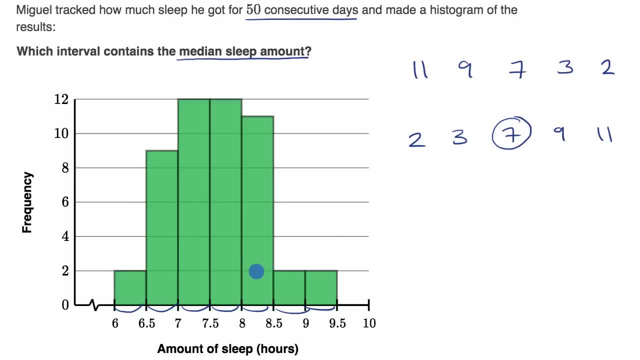 And I have a clear middle number because I have five data points. If I have an even number of data points, I still would wanna order them from least to greatest. So let's say that I have a one, one, three and a seven.